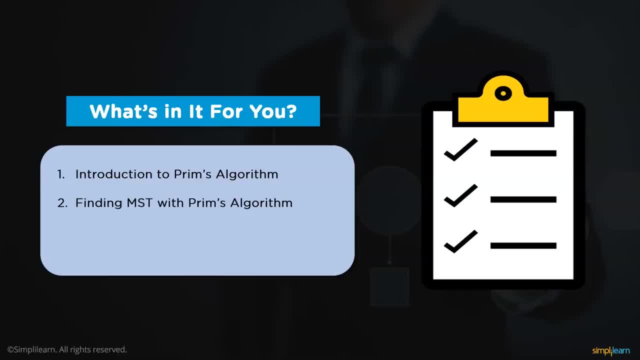 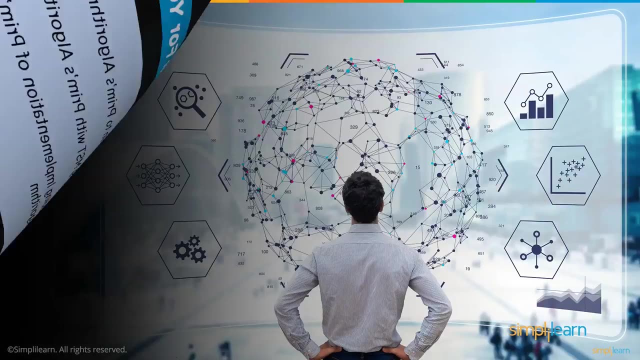 structure. Followed by that we'll deal with finding MST with Prim's algorithm And finally we'll cover the coding implementation of Prim's algorithm using C programming language. I hope I made it easy for you. Now, moving ahead, let's get started with our first topic, which is introduction to the 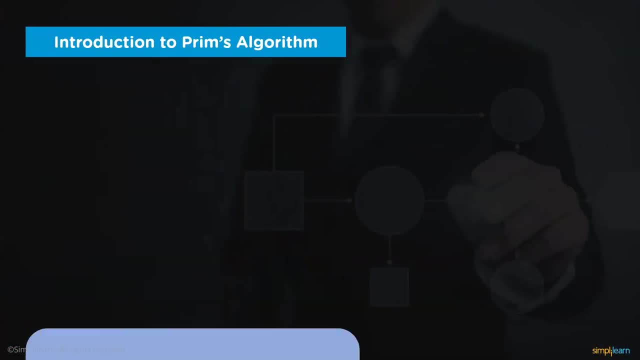 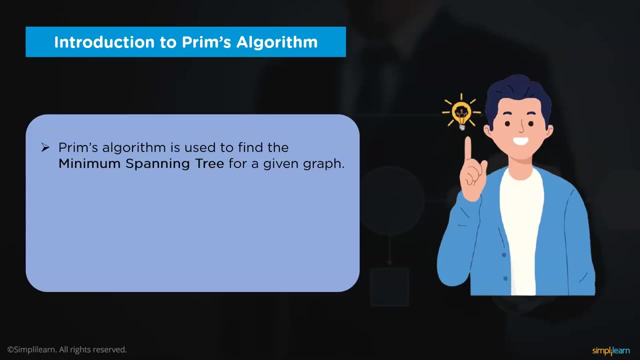 Prim's algorithm. The Prim's algorithm is used to find minimum spanning tree for a given graph. But what exactly is a minimum spanning tree, or MST? Well, a minimum spanning tree is a subset of graph G having the same number of vertices as of graph G and edges equivalent to a number. 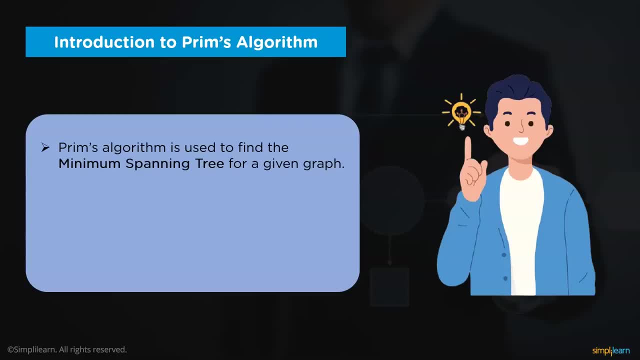 of vertices minus 1.. Along with these properties, it also has a minimum cost for summation of all edge weights included in a spanning tree. Prim's algorithm starts with a single node and explores all the adjacent nodes at every step, The edges with minimal edge weights, causing no cycles. 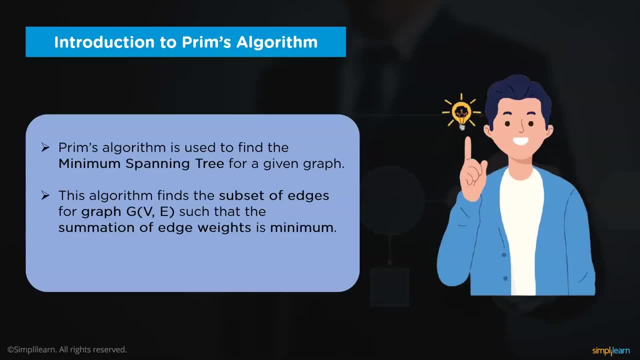 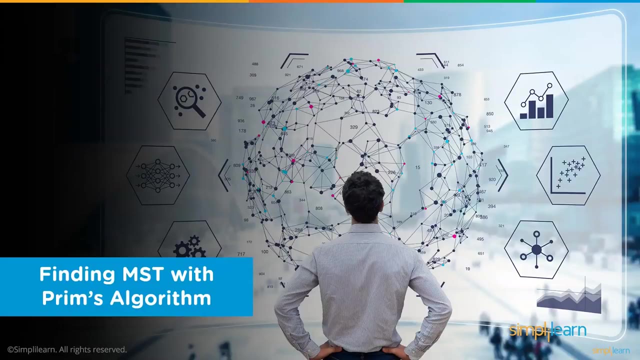 in the graph gets selected. Hence we can say that Prim's algorithm makes a locally optimal choice, intending to find global optimal choice. That is why it is called as greedy algorithm. Let's understand how we can find the minimum spanning tree using Prim's algorithm. 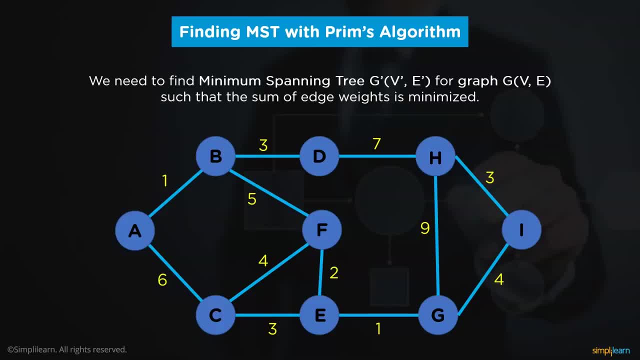 Now, given a graph G consisting of vertices V and edges E, we need to construct a minimum spanning tree G' with vertices V' equal to V and edges E' equal to V-1, having the summation of edge weights minimal. This particular graph G contains 9 vertices and 12 edges That. 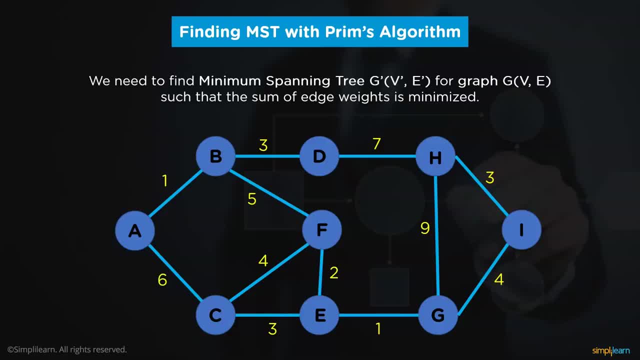 means our MST has a minimum spanning tree with all of its edges equal to V-1.. But a MST G' will have 9 vertices and 9-1 ages, ie 8 ages. So with this in mind, let's create an MST for this graph G using Prim's algorithm. 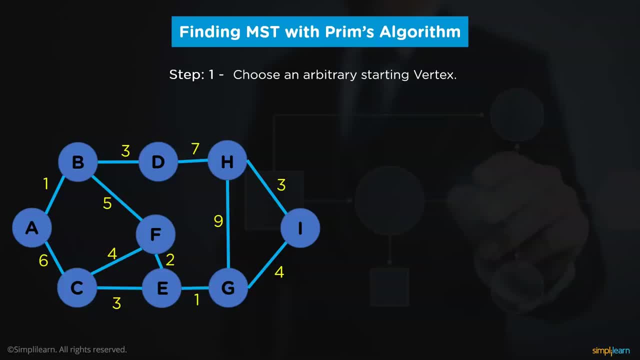 The first step in Prim's algorithm is to choose an arbitrary starting vertex. Here we'll select node A as our starting vertex. Now, the next step in Prim's algorithm is to add new vertices with a minimum age weight, In this case from vertex A. we have two possible ages for traversal. 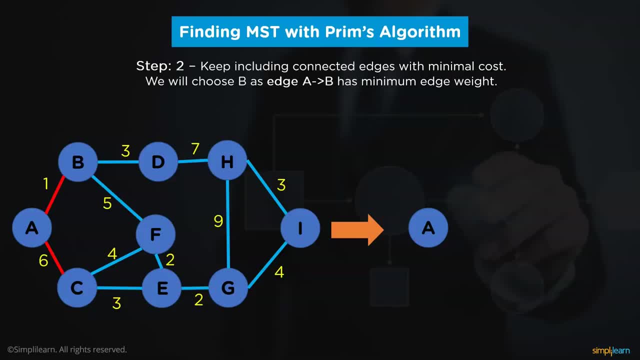 The age weight for age AB is 1,, whereas the age weight for age AC is 6.. So obviously we'll choose vertex B here. Since we have reached vertex B, we'll look into the possible ages for adding an age with minimum weight to our MST. 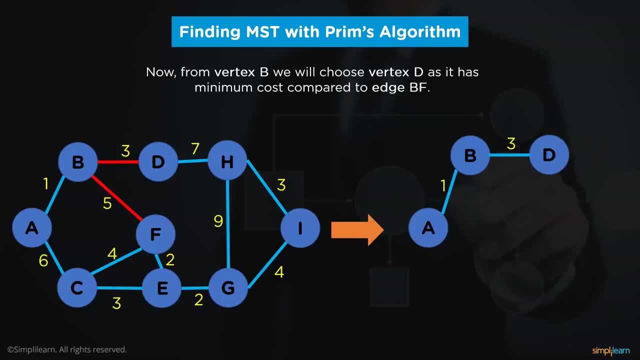 Age BD has the minimum age weight, so we'll add it to our MST Now. from vertex B we'll look into the possible ages for adding an age with minimum weight to our MST. From vertex D there is only one age, hence we'll directly add that age DH into our spanning. 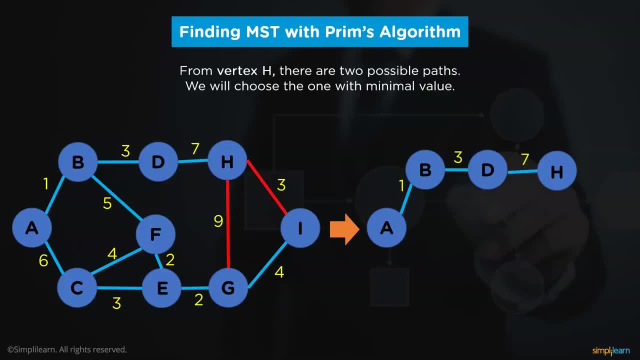 tree. Now, from vertex H, there are two possible paths, out of which the path HI has minimum cost, thus we'll add it to our MST. From vertex I, there is only one age, so we'll directly include it in our MST. 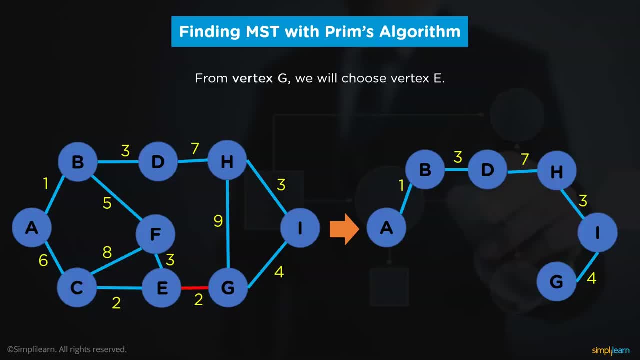 Now that I have included vertex G, I'm going to check what connected ages I have from vertex G. One age from vertex G will just insert it in our MST. From vertex E, two ages are going to different vertices, so we'll choose the one with least. 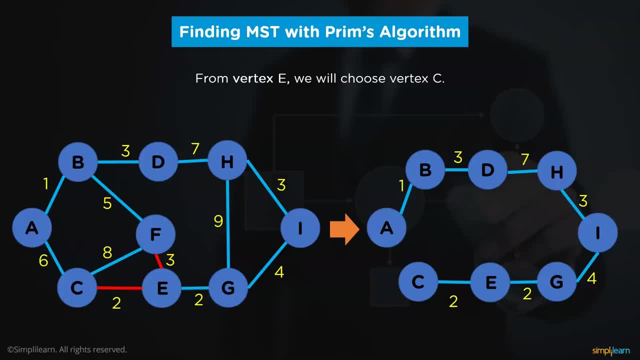 age weight, and that age is HEC. Now that I have included node C, I'm going to examine what connected ages I have to consider from vertex C. Currently, out of these two highlighted ages, I want to pick that age which has not yet been included in MST. 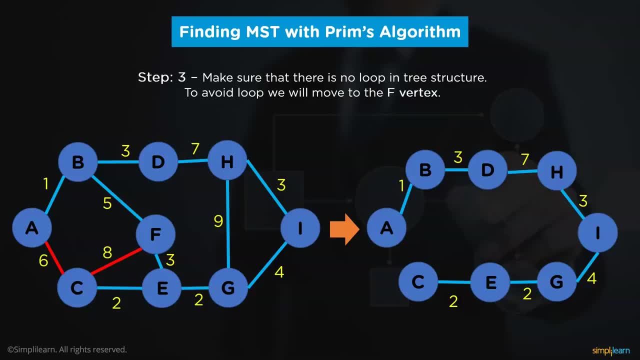 But the question that arises here is: can I add this age AC into our MST? Well, we cannot. If we add age AC to our MST, then it won't remain a tree structure due to the creation of cycle or a loop, which we cannot allow to happen according to the Prim's algorithm. 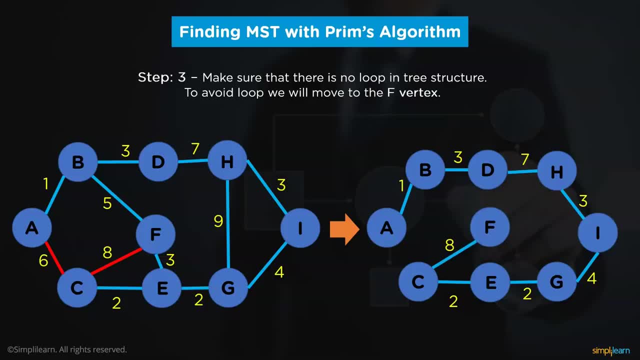 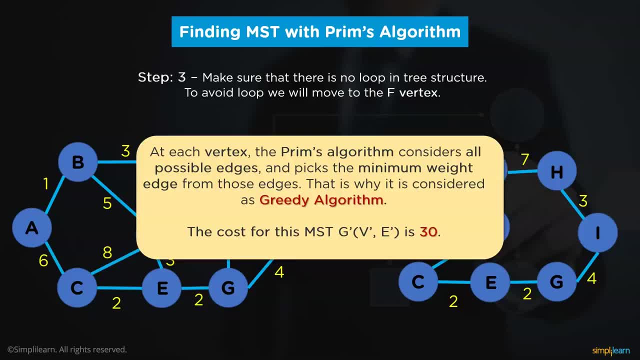 And finally the summation of age weight for insertion in our MST. Also till the time, you must have observed that this algorithm chooses the next vertex that offers the most prominent or immediate benefit. It started with an empty spanning tree for maintaining two sets of vertices. 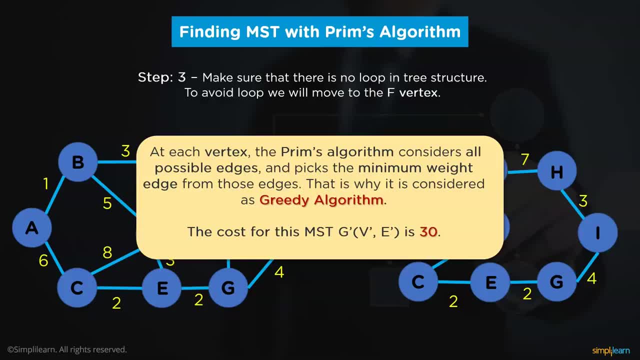 The first set was for the vertices included in the MST and the other set was for the vertices that haven't been included in the MST. At every step, this algorithm considered all the edges, that considers the second set sets and pick the one with minimum edge weight from the adjacency matrix. 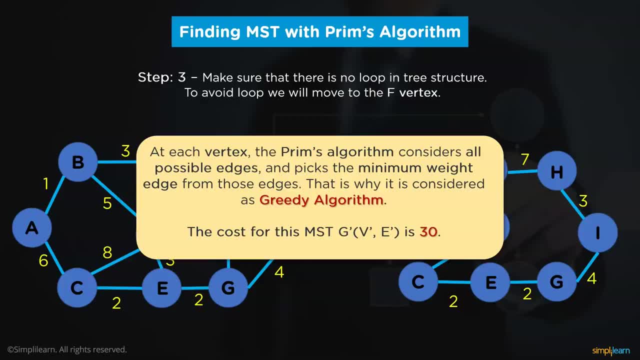 A group of edges that connects two sets of vertices in a graph is called cut-in-graph theory. So at every step of Prim's algorithm we find a cut of two sets. One contains the vertices already included in MST and the other containing the rest of. 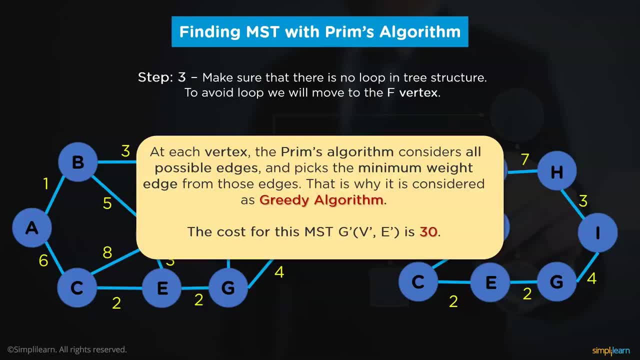 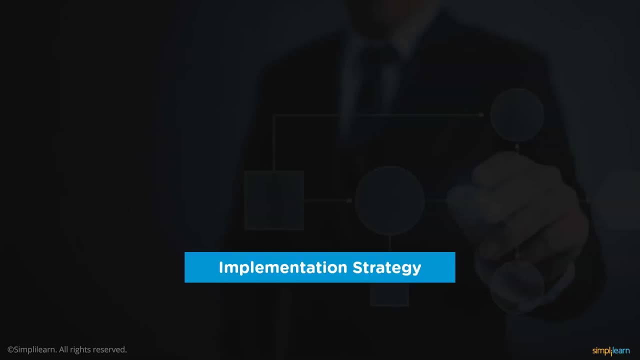 vertices. After that, we pick the minimum edge weight from the cut and include that vertex to our MST set. That is why this algorithm is called as Greedy algorithm. Having said that, let's dive into the implementation strategy for developing code for Prim's algorithm. 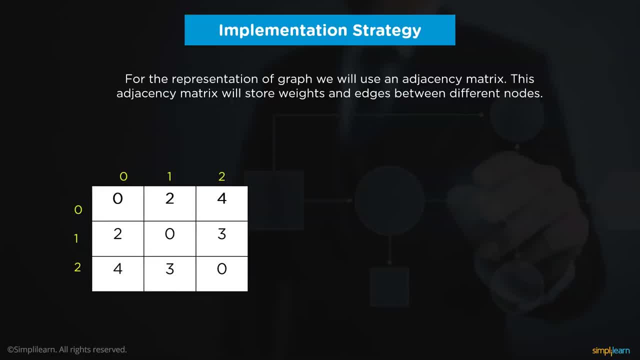 The idea behind Prim's algorithm is simple: All the vertices of a spanning tree must be connected. Hence the two disjoint subsets of vertices must be connected in order to create a spanning tree. And further, these vertices should only be associated with the minimum edge weight to. 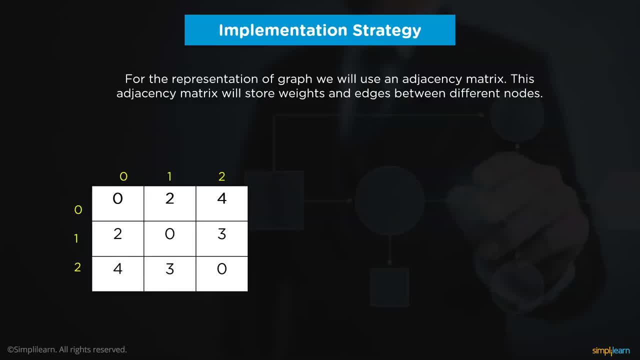 make the algorithm work, To make it a minimum spanning tree. In order to store these vertices and edges, we'll create an adjacency matrix using 2D array in C programming language. Well, the indexes of this 2D matrix will be the vertices where the values other than 0. 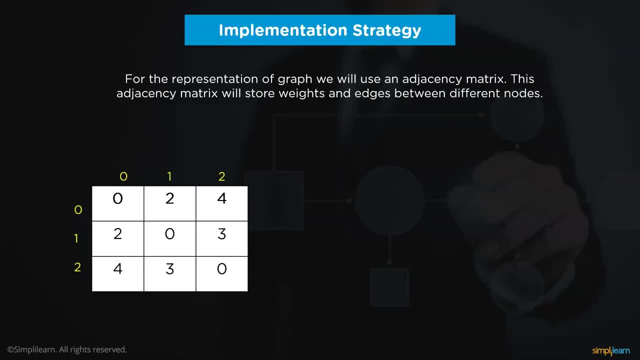 will be the edge weights For indexes 0,, 1 and 2, you can clearly see that the adjacency matrix is having value 0. That means there is no recurring connection or loop for these vertices, so primarily, let's add them to our graph structure. 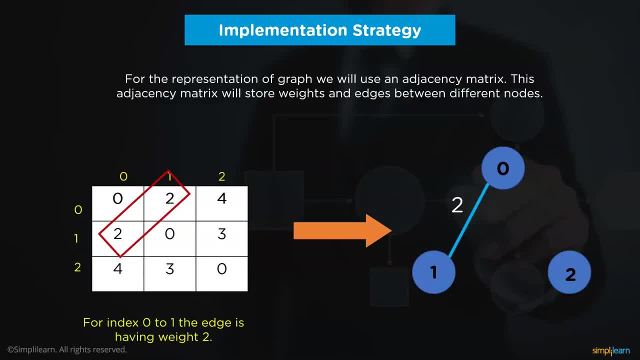 For edge 1 to 2, we have the weight value 2.. So we'll add edge between vertex 0 and 1.. After that we have edge between 2 and 1. The value for this edge weight is 3.. 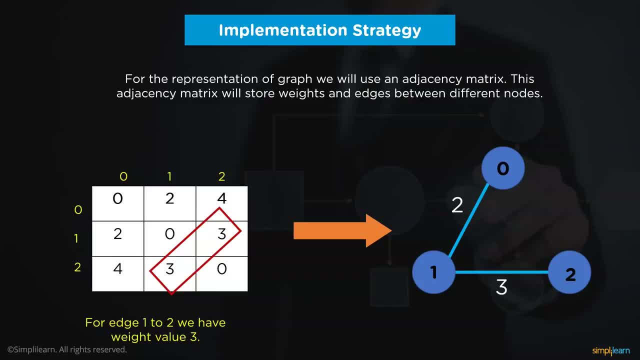 So we'll add edge between 1 and 2 and assign 3 as its edge weight. Finally, the edge weight for connecting 0 to 2 is 3. So we'll insert it in our graph as well. In the next slide we'll discuss the strategy for implementation of a prims algorithm. 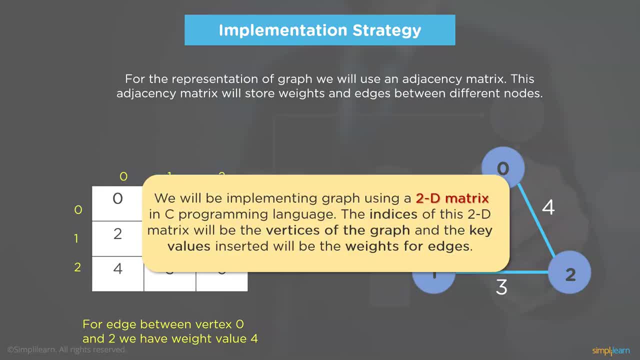 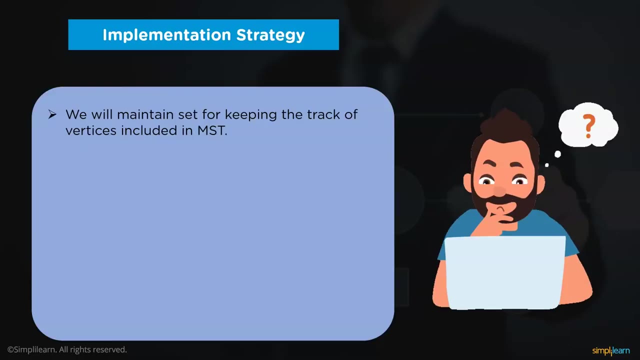 From this example, I hope you are clear with how we are going to maintain a structure of a graph using 2D matrix. In the next slide, we'll discuss the strategy for the implementation of prims algorithm. The first step of this algorithm is to maintain a set for keeping track of vertices included. 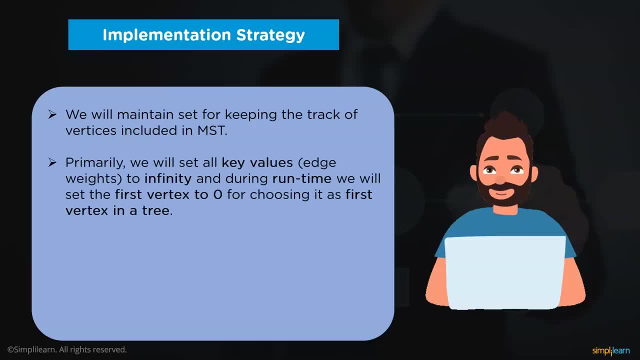 in an MST To create the set. we'll assign a key value to all vertices in the input graph. Initially we're going to set all key values as infinite and at the runtime we'll assign weight 0 to the first vertex. 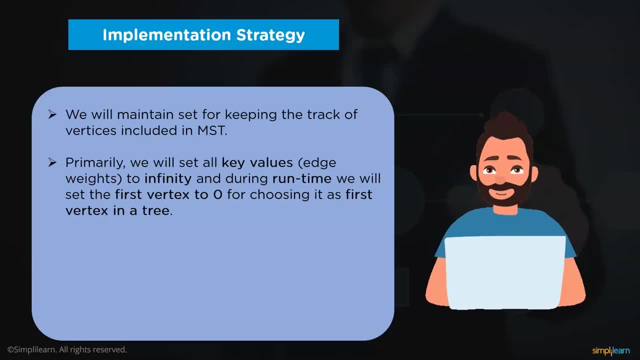 By doing that, we choose it as an arbitrary starting vertex. Once done with that, we'll start adding vertices to our minimum spanning tree. For that we'll pick up a vertex u with minimum weight to insert it into our set. After that we'll also update the key values for all vertices. For that. we'll pick up a vertex u with minimum weight to insert it into our set. After that we'll also update the key values for all vertices. So we'll create a set for keeping track of vertices included in the MST. So we'll create a set for keeping track of vertices included in the MST. 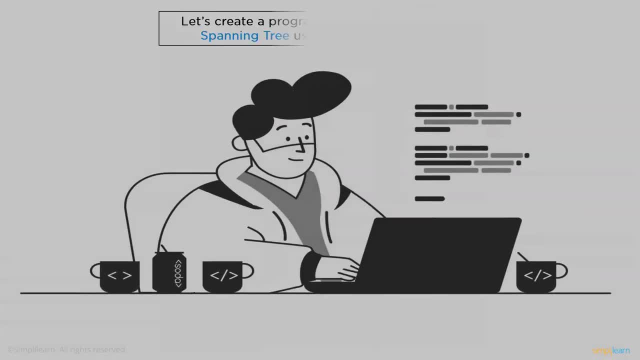 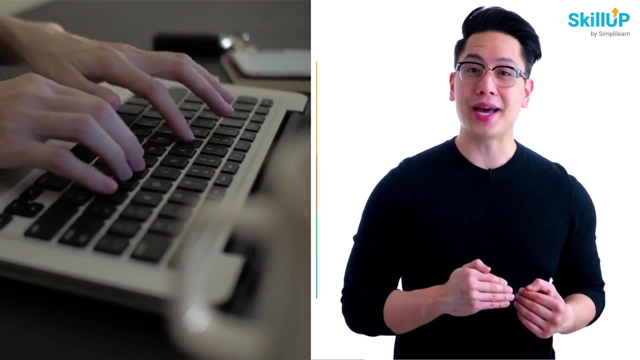 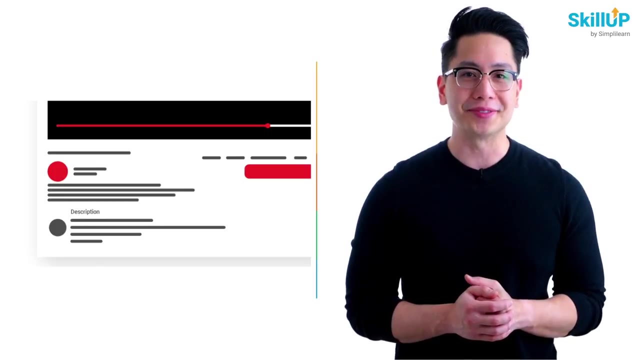 On that note, let's visit a code editor to implement prims algorithm using C programming language. If getting your learning started is half the battle, what if you could do that for free? Visit scaleup by simplylearn. Click on the link in the description to know more. 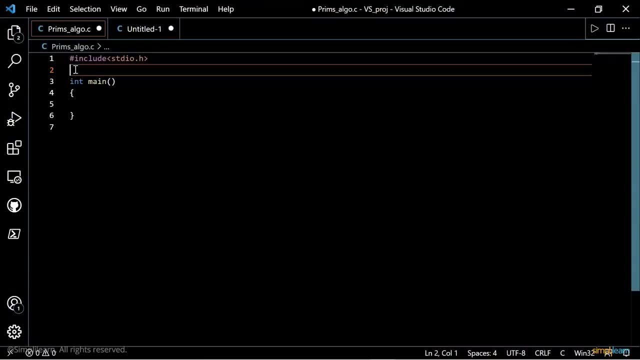 Now, in order to begin with coding implementation, we'll need to load some dependencies For this implementation process. we are going to need a Boolean set in order to keep track track of vertices included in our msd. that is why we'll include a standard boolean library in our 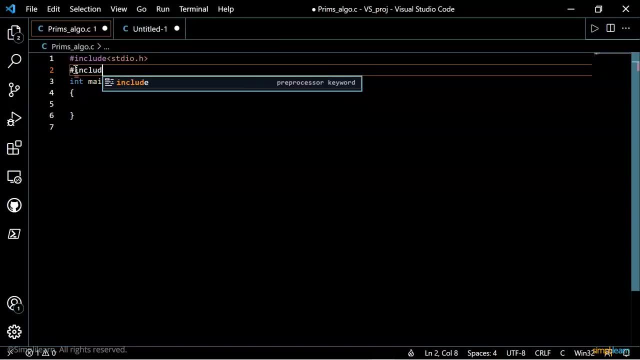 program. so hash include std dot edge. once done with this addition, we'll define a number of vertices that we are going to use in our graph. i am going to set the number of vertices to 5, so let's do that. hash define vertices 5, and if you want to implement mst for a larger graph, then you must set the number of vertices. 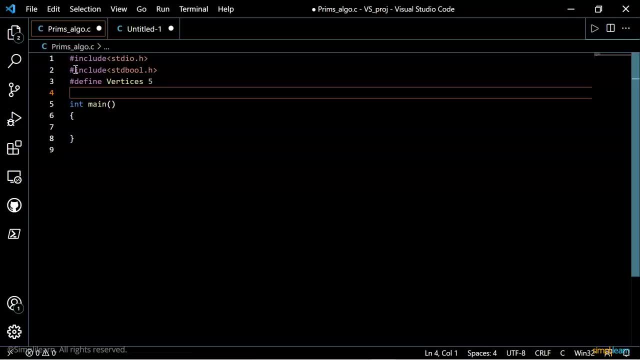 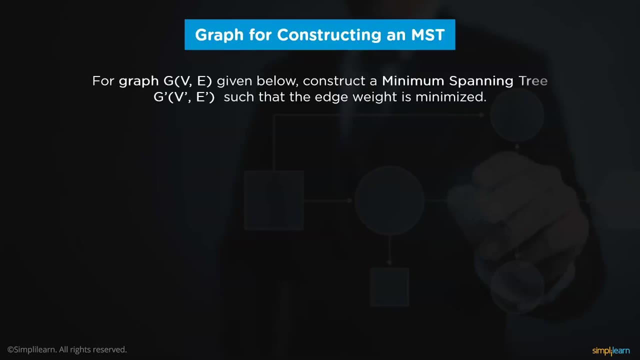 to a more significant number. Now let's move to the main function. The graph that I am going to use for generating a minimum spanning tree is supposed to be stored inside a 2D matrix, So first let's have a look at that graph. 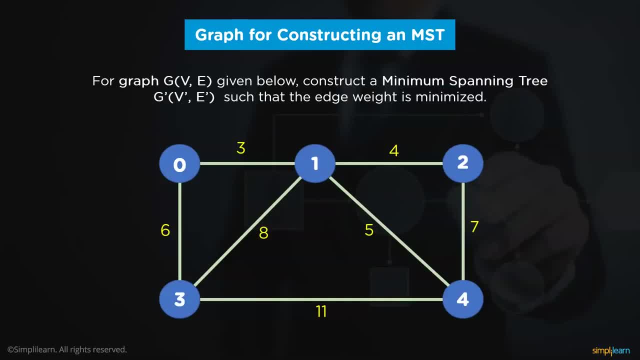 This is the graph for which we want to develop a minimum spanning tree. The first step that we must take to do that is converting this graph into 2D matrix, As discussed earlier. the diagonal values will be null or zero and other values will be the. 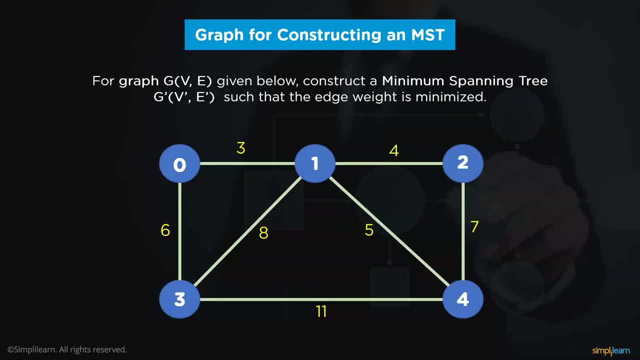 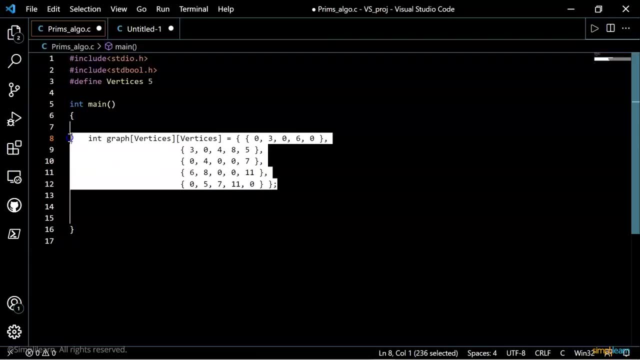 edge weights between two nodes. So, without wasting any time on this, I will directly create adjacency matrix for this graph inside our code editor. This part is about maintaining our graph in form of 2D matrix. Now, after this, we are calling prims mst function, which is responsible for generating a minimum 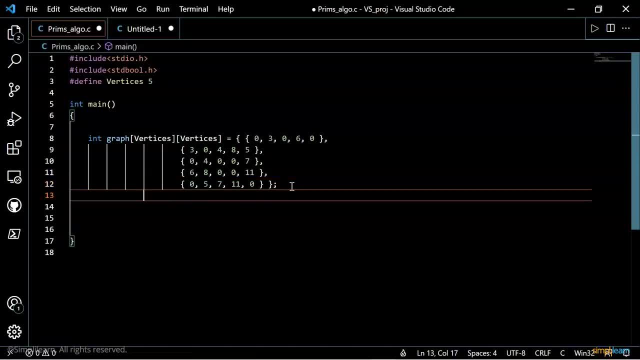 spanning tree. So let's do that here. So let's create prims mst function, void prims underscore mst, and we'll pass this graph to this function. But we haven't developed any code for this prims mst function. but we'll do that now. 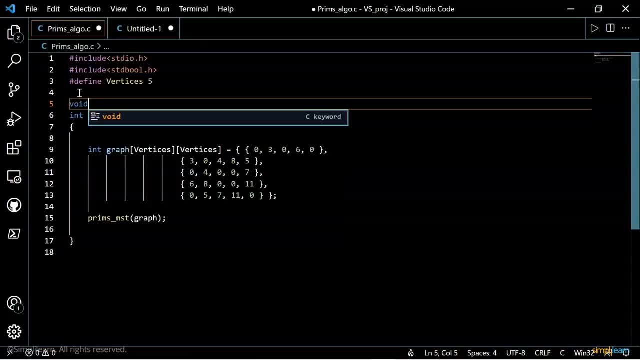 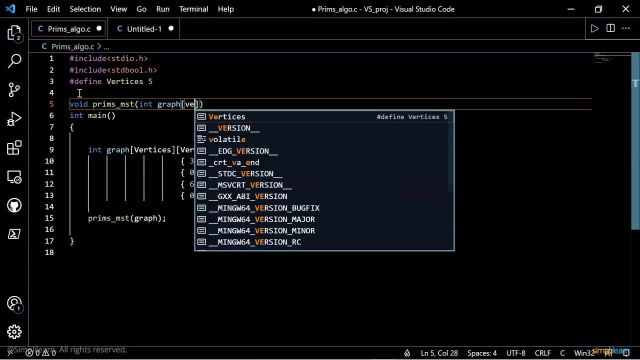 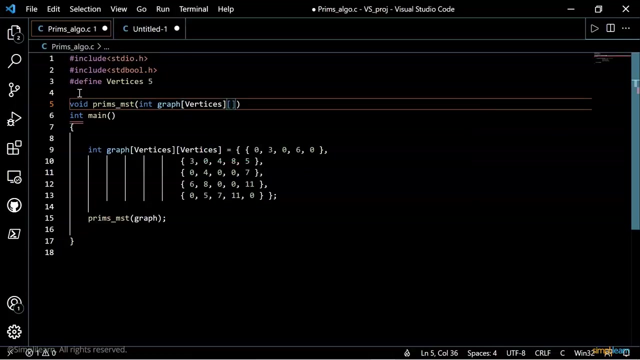 So let's create prims mst function. void prims underscore mst- Okay, And we'll pass graph as an argument should be vertices and vertices to make it a 2D matrix. Now, inside this function we'll create an array named key to store key values of all. 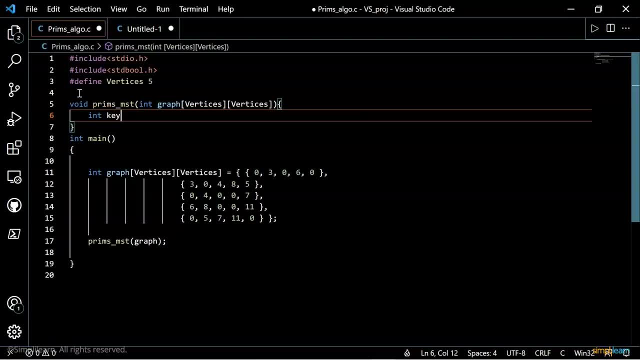 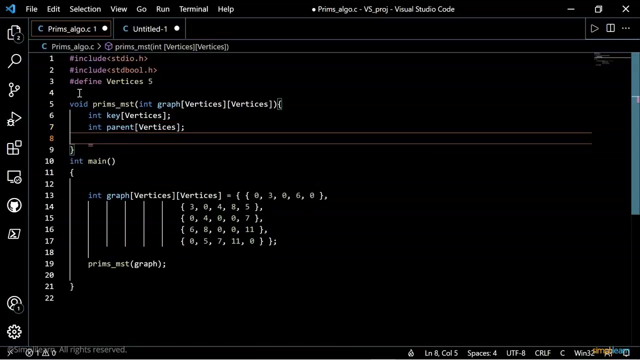 vertices and key vertices. Along with it, we'll also initialize the parent in which we'll store our actual mst and Boolean set to keep track of each and every vertex of our graph. So let's create that parent array. We'll create an array named key to store key values of our graph. 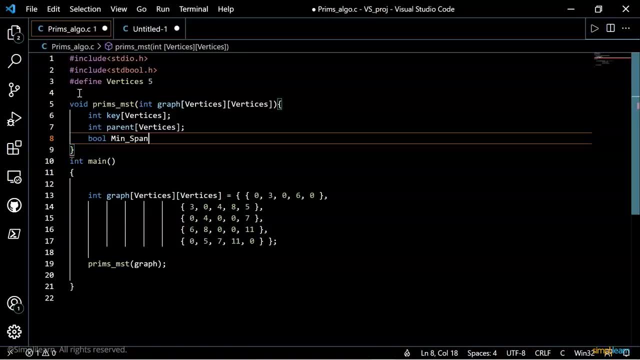 And we'll create an array named key to store key values of our graph, And we'll also initialize our hash data to keep track of all vertices And we'll create Boolean set for maintaining track of all vertices. Okay, Now, after this, what we'll do is we'll set the key values of all vertices to infinity. 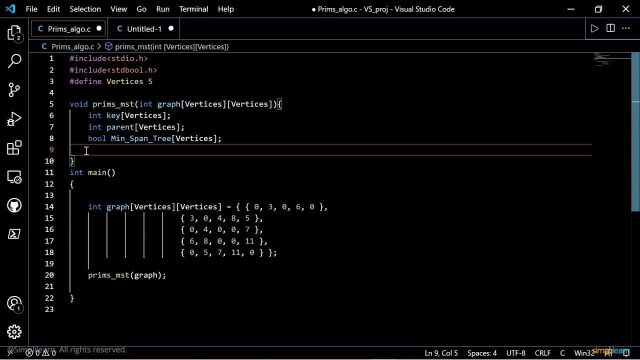 and we'll also make sure that these vertices are not part of our minimum spanning tree set. so for that we'll create a for loop and inside this for loop we'll use iterator element I and will initialize this element to zero till vertices and will increase the iterator element I for each loop. 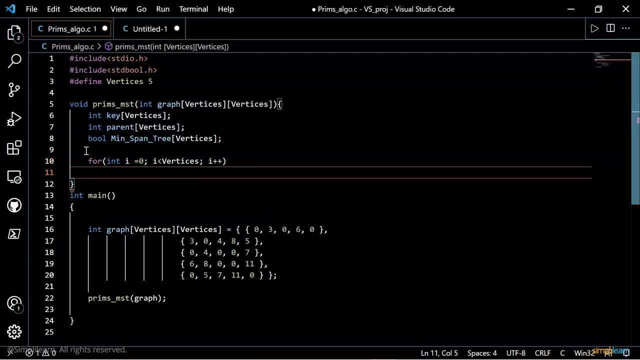 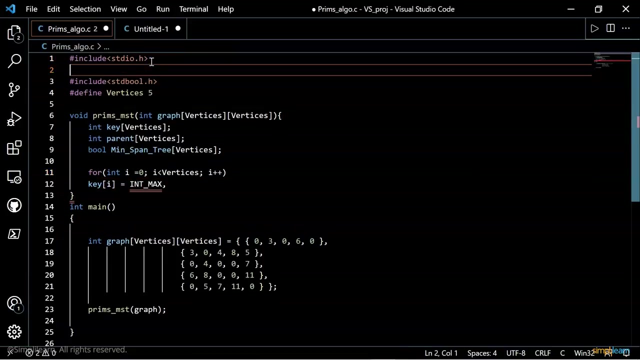 inside this loop we will set key I for interceptados to the possible integer maximum value and in order to use this value we'll need to add one library, which is called as limits, dot H. so we'll add it here. hash include limits, dot H. okay, after. 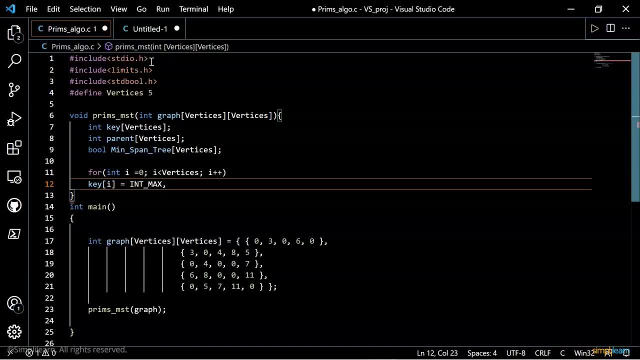 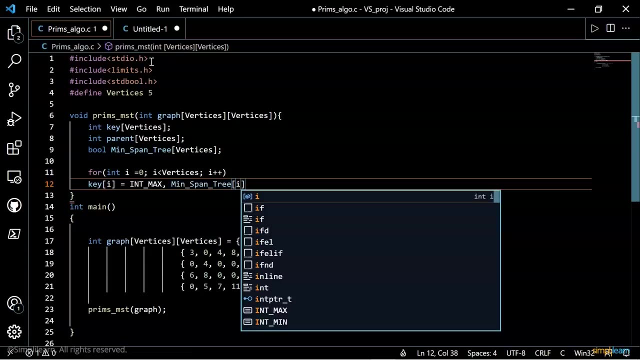 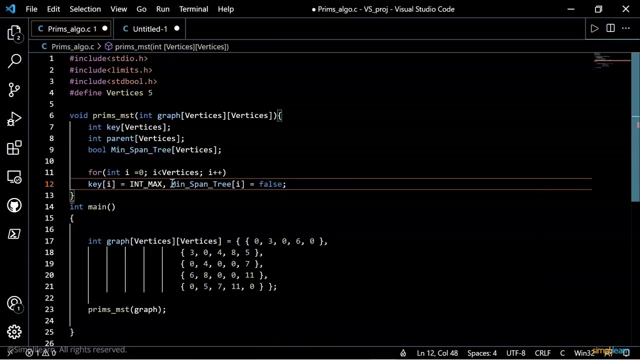 this. we will also make sure that these vertices are not part of our minimum spanning tree set or Boolean set. so for that we'll write statement mean underscore span, underscore tree. I should be false. that means empty and we'll add indentation. okay, now, in order to choose, the arbitrary index will set the key value of a first. 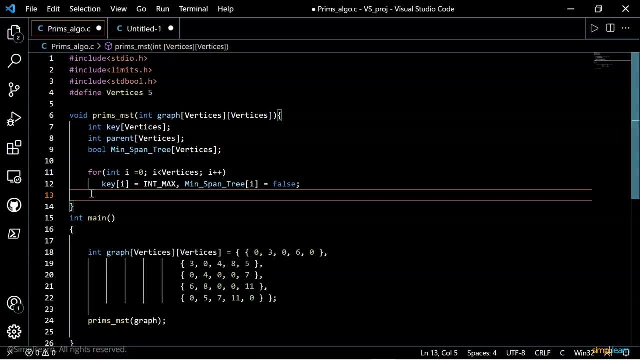 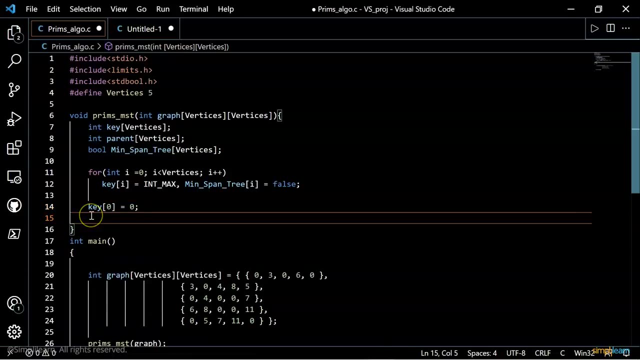 vertex to 0, so that it will be chosen first in our minimum spanning tree. for that we'll write statement key 0 should be equal to 0 and as we have chosen vertex 0 as our first arbitrary vertex, so we'll also set the index 0 of the 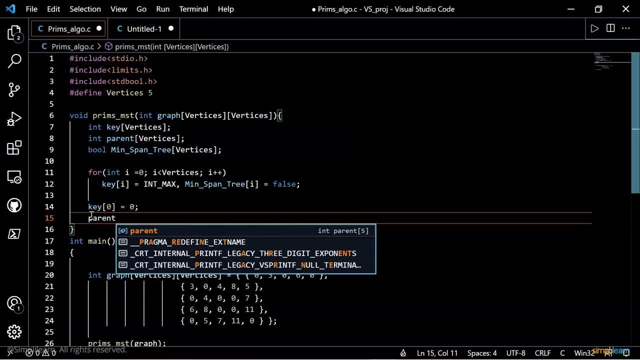 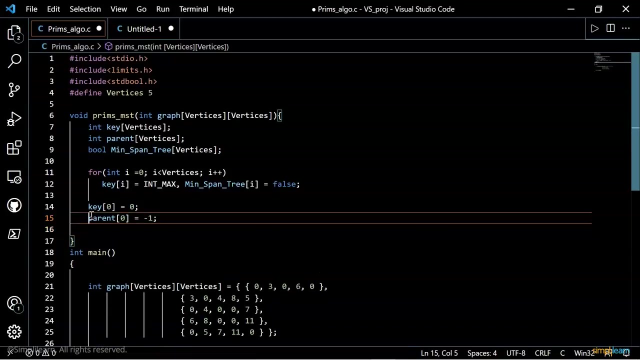 parent array to minus 1.. By doing this, we are ensuring that the index 0 is the root node of our minimum spanning tree. Now, to choose vertices with the minimal key value, we will create a new function named least key. So let's do that. 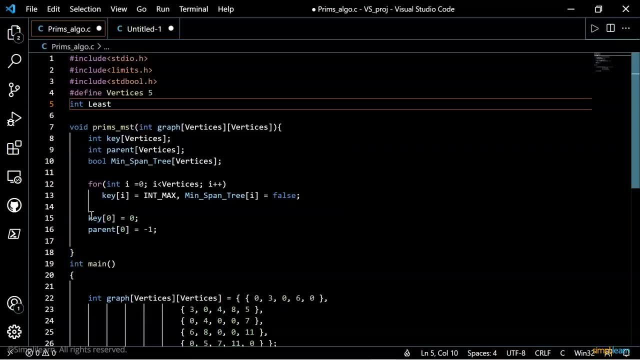 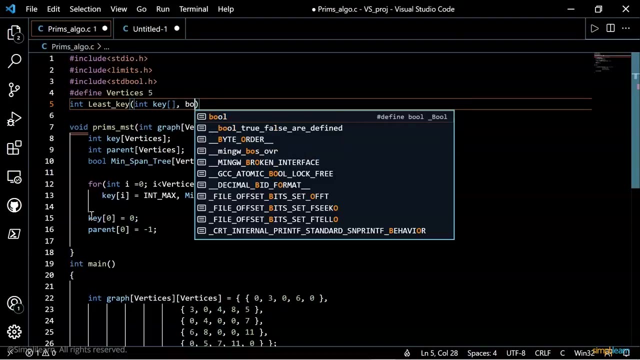 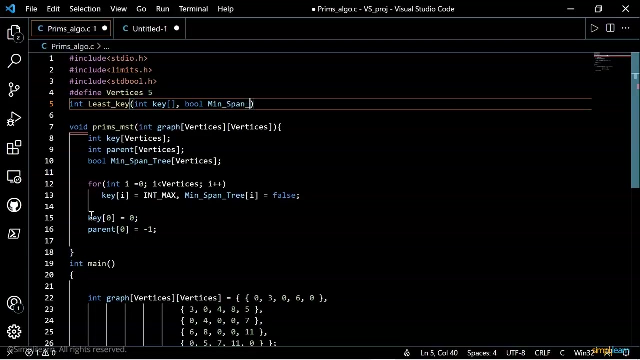 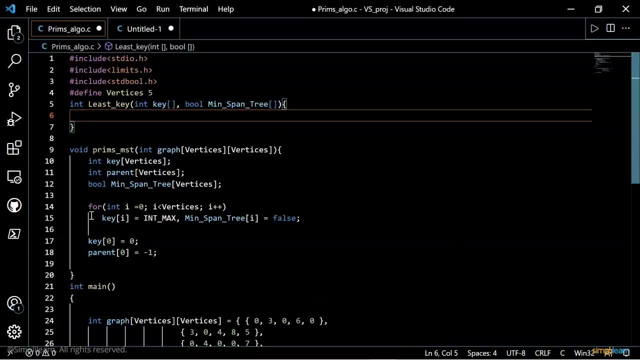 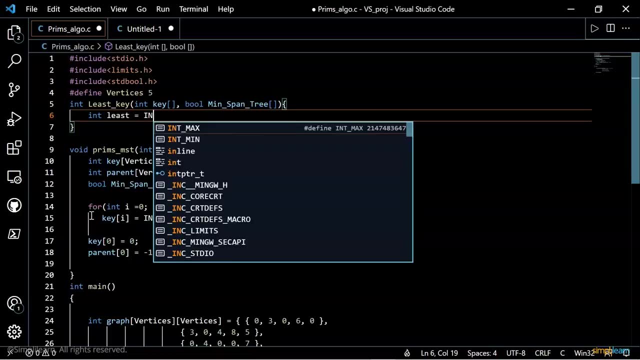 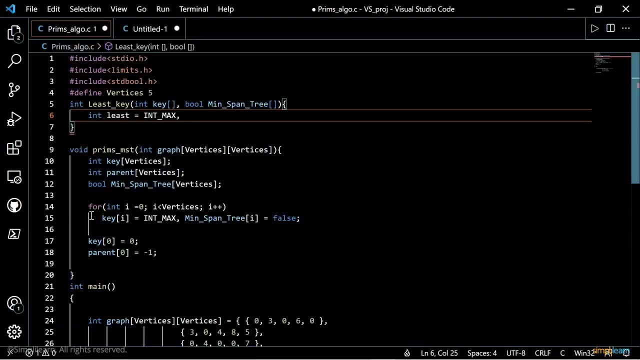 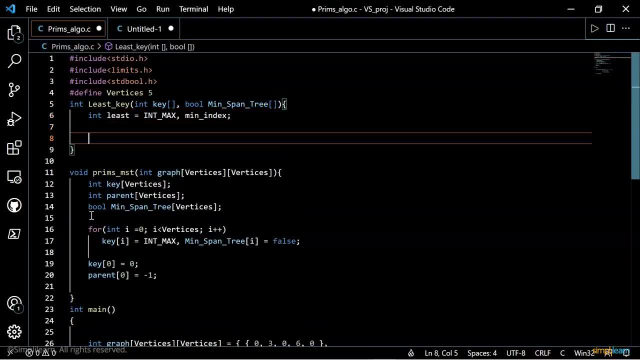 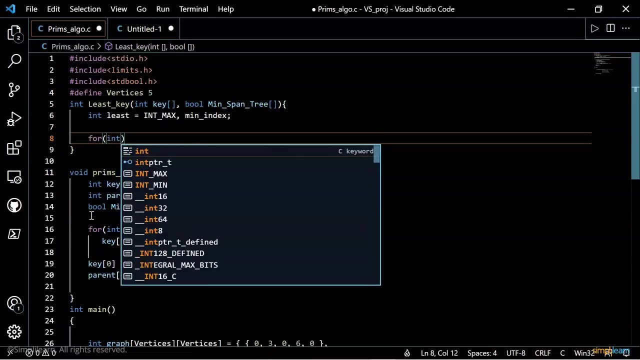 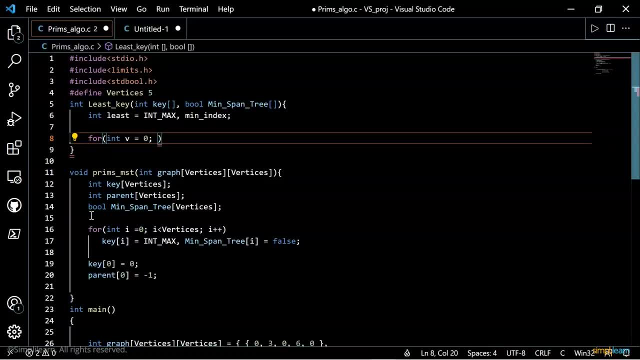 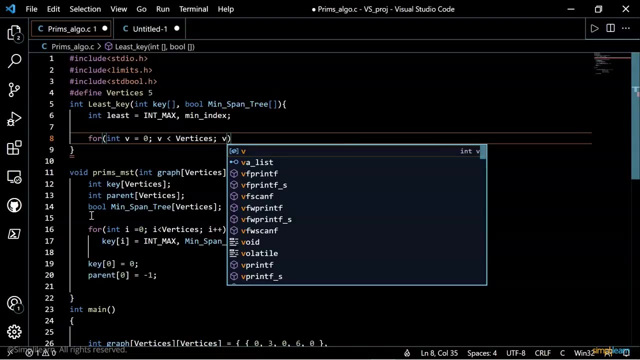 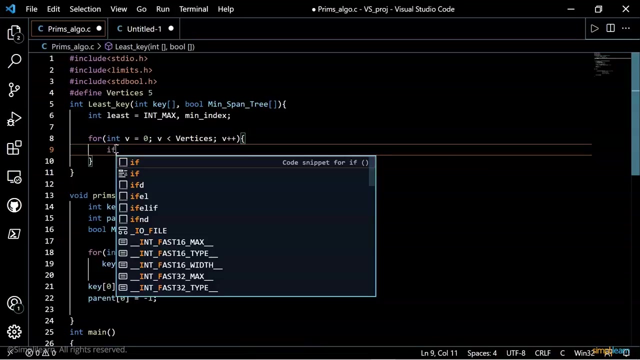 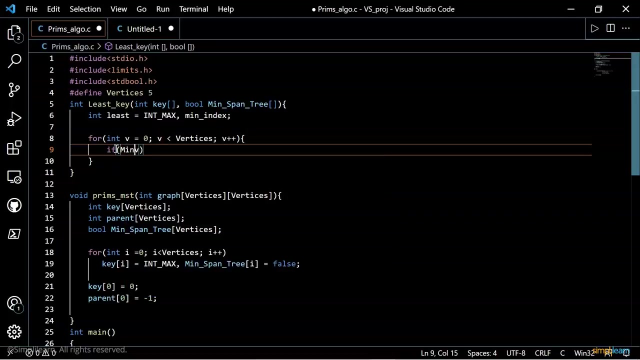 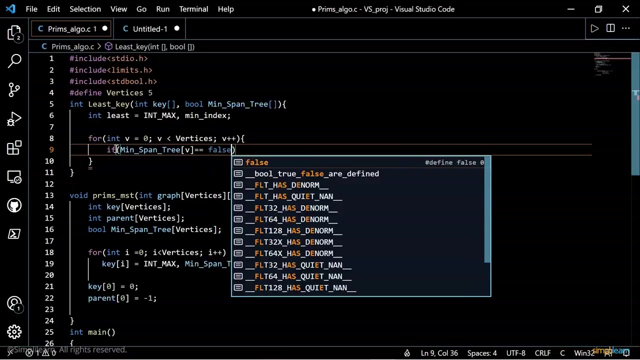 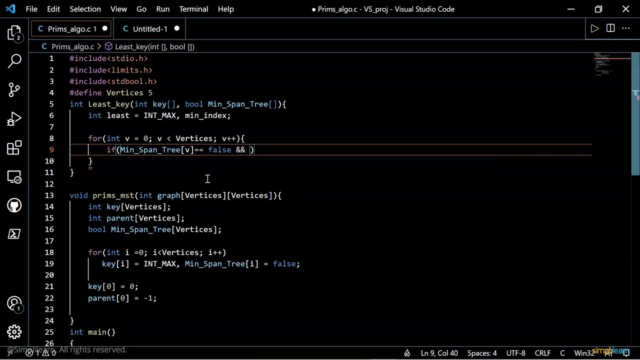 it to value 0 and the maximum limit for this v will be vertices and will increase the value of this small v variable plus plus. now, if the chosen vertex is not present inside minimum spanning tree set and then the key value for that vertex is also smaller than list. 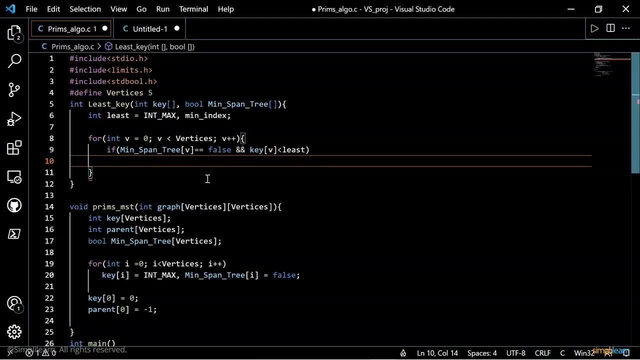 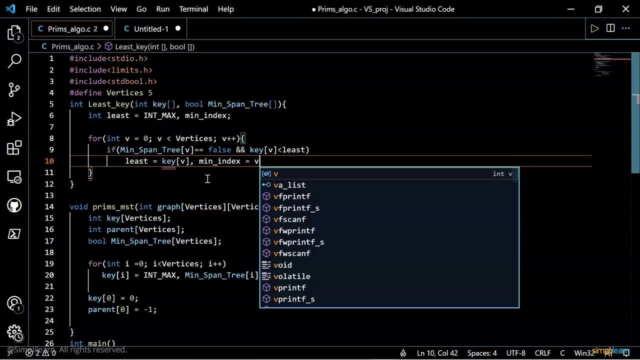 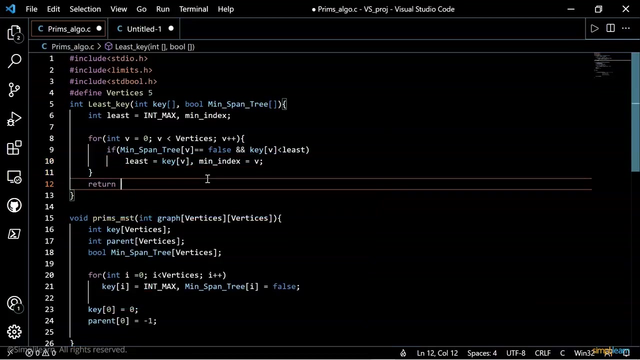 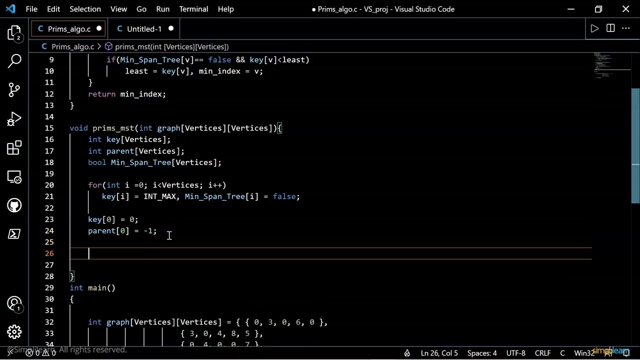 then we will set least equal to key of v and minimum index to v and we'll get out of this for loop and we'll return the minimum index value. on that note, let's arrive back at our prims msd function that we have created here. using a for loop, we'll fetch the minimum index that we have generated inside our list key function. 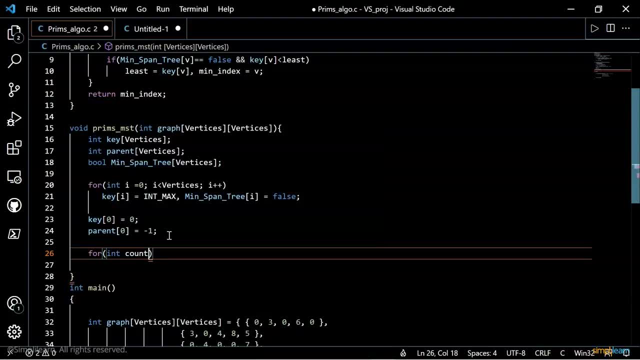 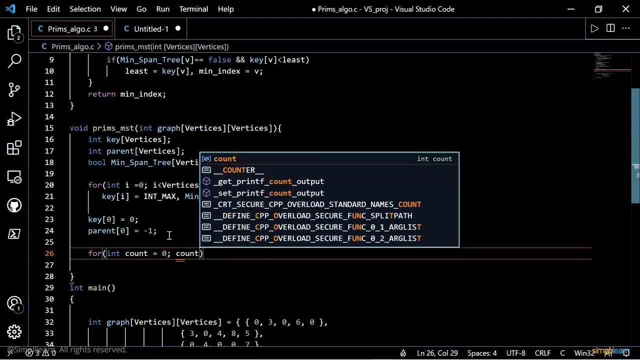 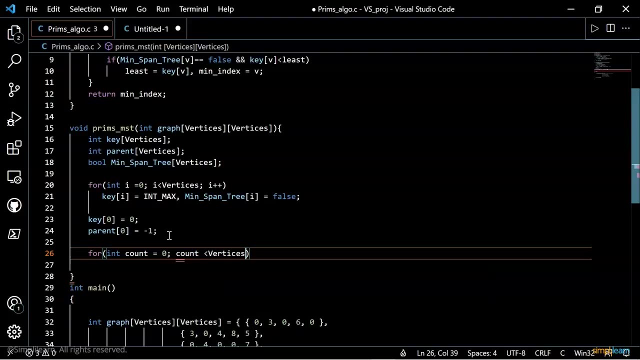 so let's create for loop. we'll use count variable here and we'll initialize it to zero. and we'll move this count variable till vertices 1, which is nothing but the number of vertices in our minimum spanning tree. next we'll increase this count variable. now we have arrived inside this for loop body. now we will store that fetch. 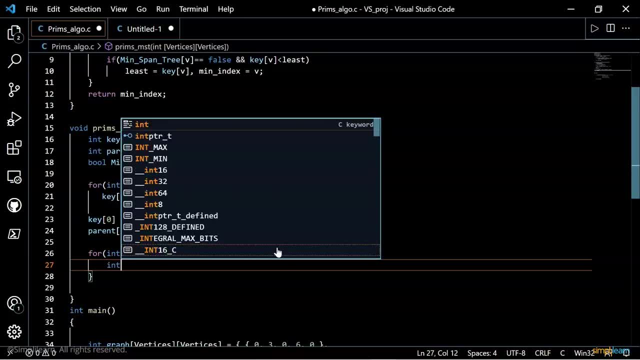 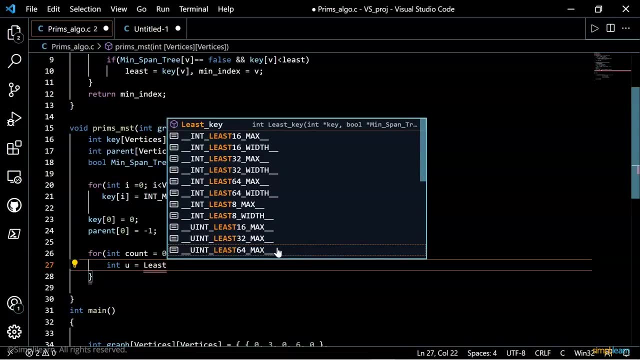 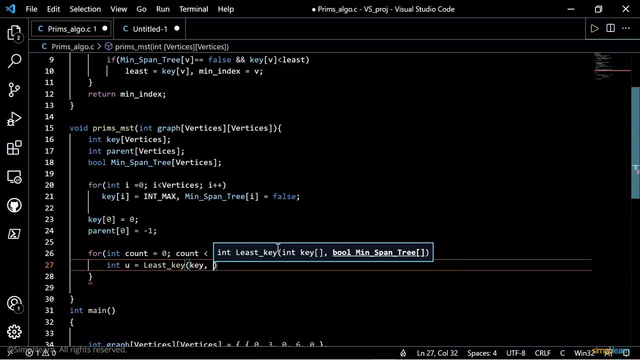 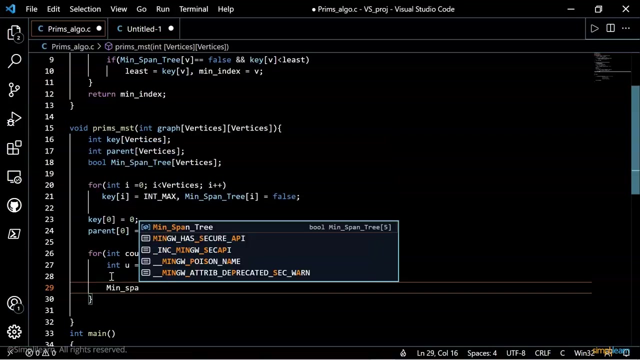 minimum index value in variable you, so in you will be equal to least underscore key and will pass key and boolean set, that is mean underscore span, underscore tree, and we will include this least node, that is, you, to our minimum spanning tree set or boolean set equal to true. 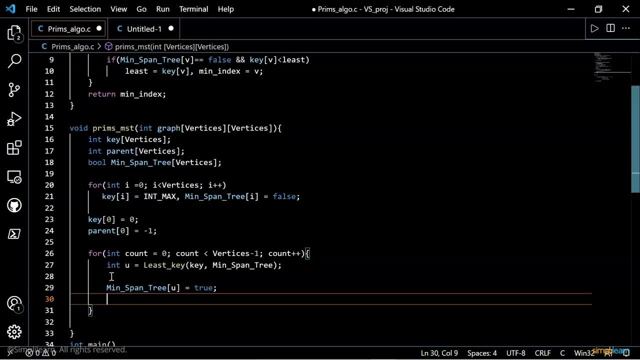 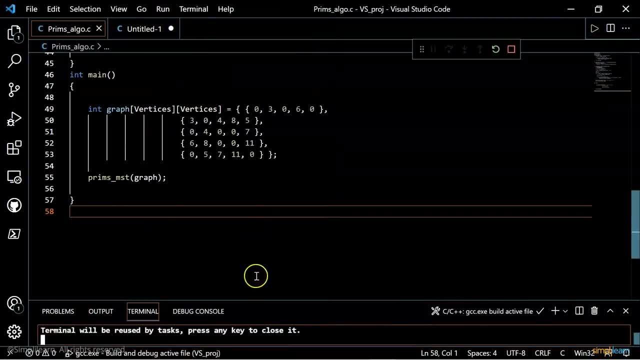 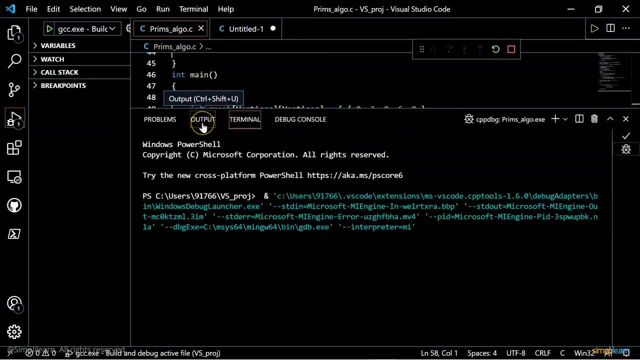